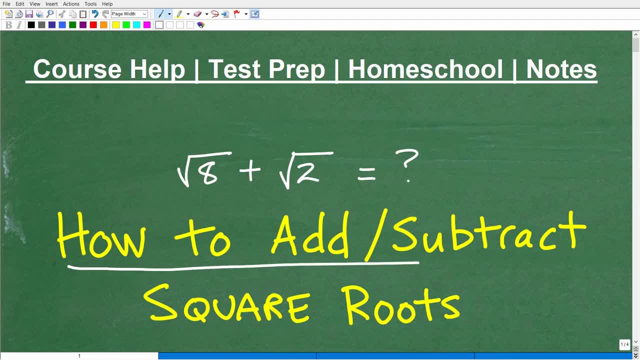 Okay, let's talk about how to add and subtract square roots. So what am I talking about exactly? Well, I'm talking about dealing with problems like this: We have the square root of 8 and we would like to add it to the square root of 2.. So what is the answer? Now notice: I said that we 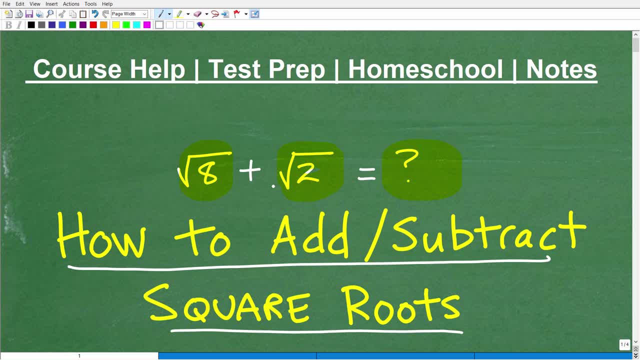 would like to add these up. Sometimes, when you're adding or subtracting square roots, we can't really simplify the expression. You'll see why here in a second. But what I'm not talking about is getting our calculator out and typing in the square root of 8 and getting some decimal, and then 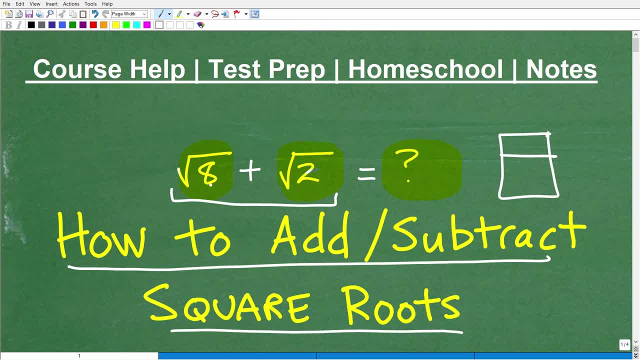 typing in the square root of 2 and getting some decimal and adding those two up. That's not what I'm talking about. So let's put our calculators away, except for the one between your ears. That one comes in pretty handy. So if you know what to do here, go ahead and type in your answer. 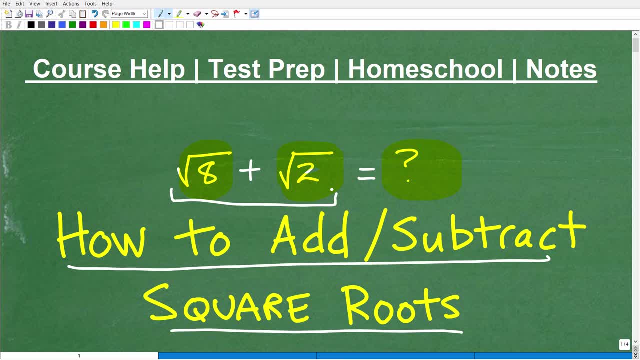 into the comment section, because this is absolutely essential skills in any sort of algebra course. Okay, so I'm going to get to exactly what we need to do to add and subtract square roots in just one second, But first let me quickly introduce myself. My name is John. I'm the founder of Tablet Class Math. I'm also a middle and 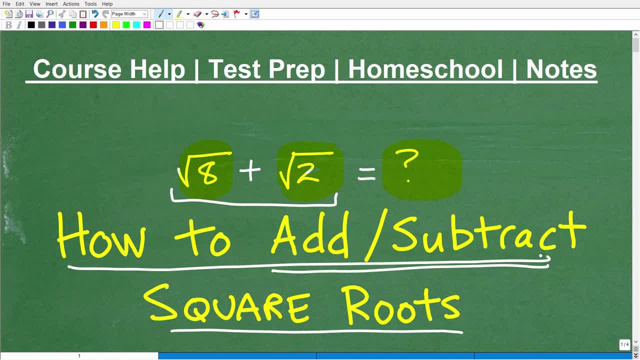 high school math teacher. I'm going to leave a link to my math help program in the description of this video. But I've been teaching math for decades and I really kind of developed a teaching style where I really explain things in a super clear and understandable way. so anyone and everyone. 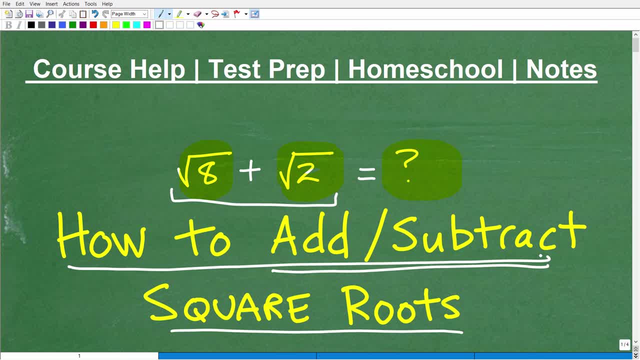 can learn mathematics, and anyone and everyone can learn math. So let's get started. I'm going to show you a very simple method to learn math. As long as you're willing to do your part, I think I have the right instruction for you. So if you're at the middle school, high school or college level and you need assistance in mathematics, definitely check out my math help program. 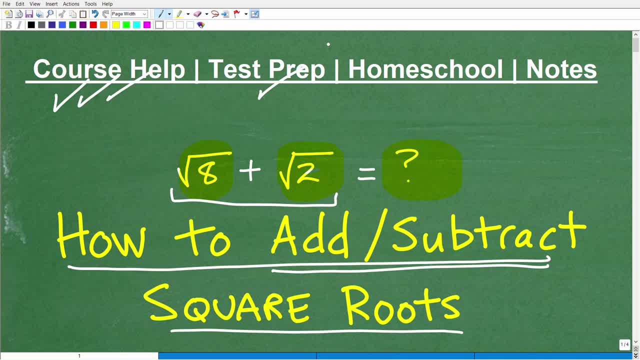 So if you're at the middle school, high school or college level and you need assistance in mathematics, definitely check out my math help program, But I'm also going to leave a link to my math help program in the description of this video. So let's get started. 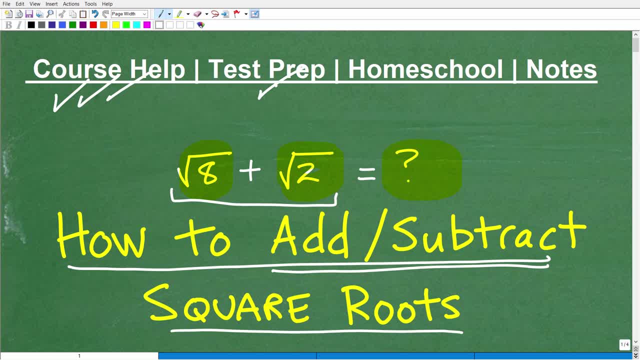 exam, But I'm also talking about tests like teacher certification exams and maybe nursing school entrance exams or the ASRAP or the military- all these different exams. I have test prep courses so I can help you prepare and pass those exams If you homeschool. I was just 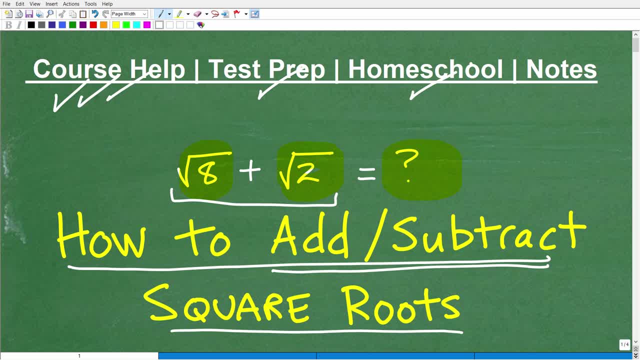 recently voted my middle and high school math courses number one for homeschooling by a major homeschool publication. Pretty excited about that And if you need some math notes, I'm going to leave links to my math notes in the description of this video. Okay, so let's get into how to add. 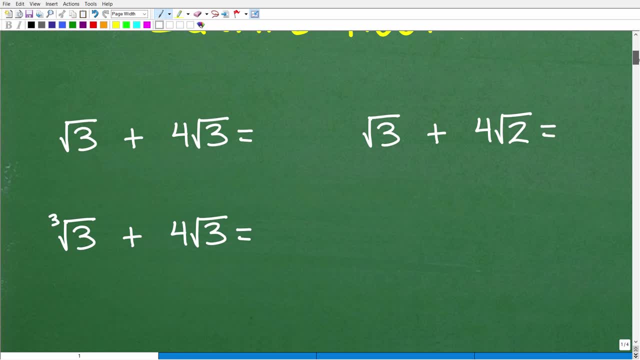 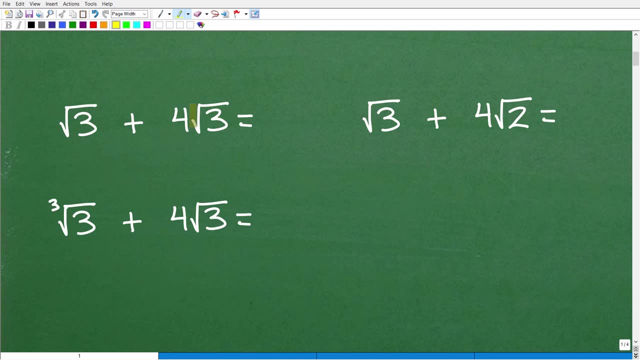 and subtract square roots. So let's take a look at some basic examples and we'll get back to that example here in a second. So let's take a look at the square root of three plus four times the square root of three. So what is the answer? I'm going to go ahead and tell you the answer, The. 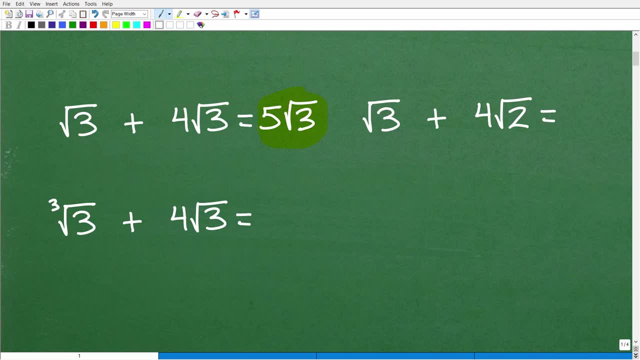 answer is five times the square root of three. Okay, so how did I get that answer? So here you have the square root of three, but outside right, here you really just have one square root of three or one times the square root of three. So this is just one square root of three, And then 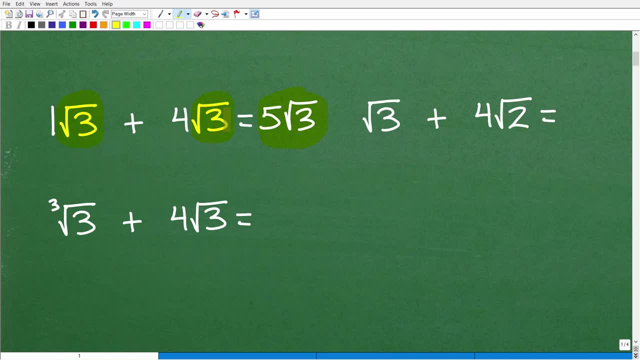 over here. I have a square root of three, but I have four times the square root of three. So this is like having four square roots of three. So if I have one square root of three over here and I have four square roots of three over here, okay, let's kind of look at it this way. right, This is. 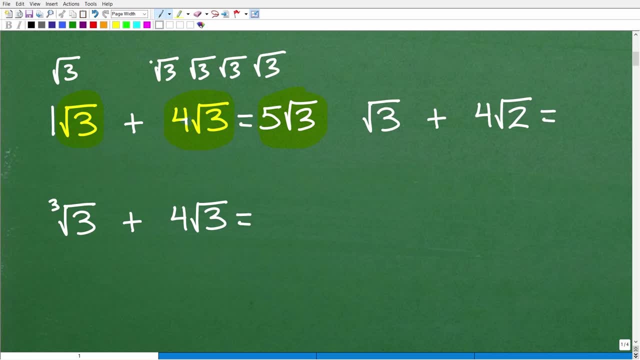 square root of three. that means that you have four square roots of three. so here I have four square roots of three, I have one. all together, collectively, we have five square roots of three. let's take a look at this right here, this problem, in another way. I want you to think of this square. 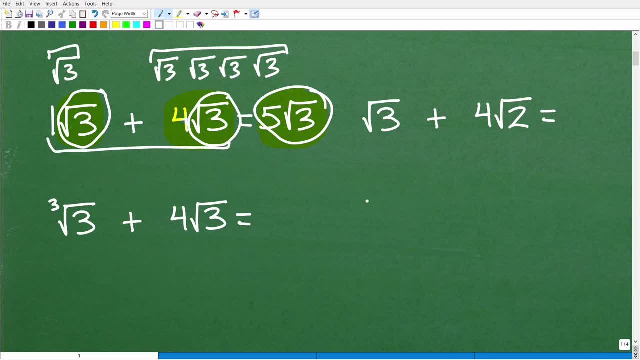 root of three and a square root of three like a variable. so here let me just write it this way: we have one square root of three plus four square root of three. I want you to think of these here kind of like a variable. if you're familiar with how to add like terms, let's 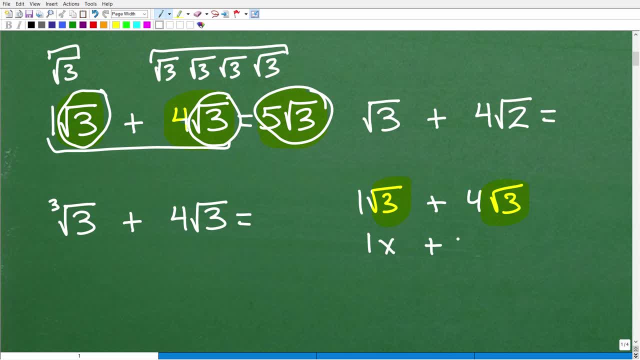 replace the square root of three with x, so I just have one x plus four x. so how many x's total do we have? we have five x's, okay. so as long as you have the exact same square roots, okay, in other words, square root of three and the square root of three. we simply just add these numbers here. okay now? 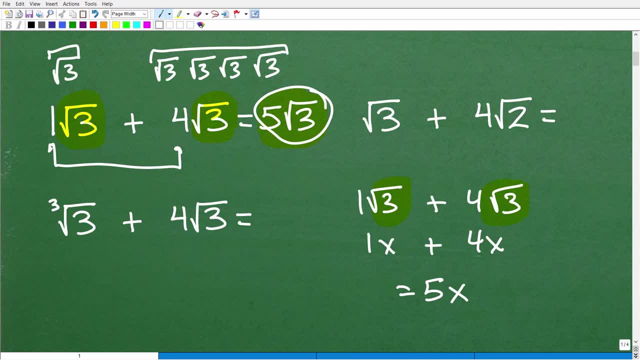 these numbers, the one and the four. these can be positive answer, negative numbers. so, whatever, these are the sum of these numbers. you're going to put that in front of the square root of three. okay, so let's take a look at some other problems here. so we do not. 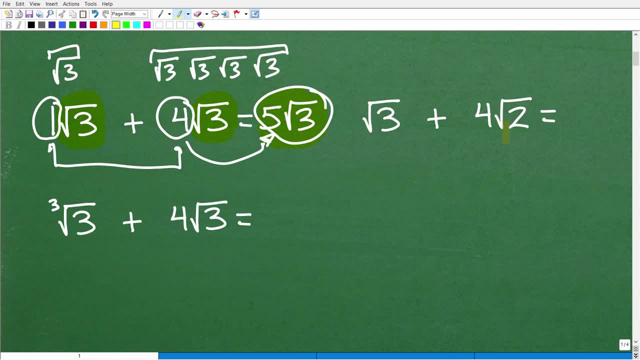 confuse this rule. so how about the square root of three plus four times the square root of two? how do we add these up? well, i have a square root of three here and i have a square root of two here. okay, can i? are these exactly the same? can i add these up? no, you cannot, because this, this is a. 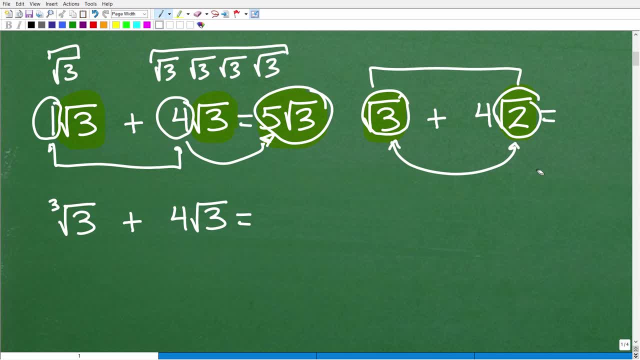 square root of three and this is a square root of two. we cannot add these up. so, to kind of use my algebra example, the square root of three, this might be like x, and then this is like this is a different variable, like four times y. so these are different. okay, so, in order to add or subtract, 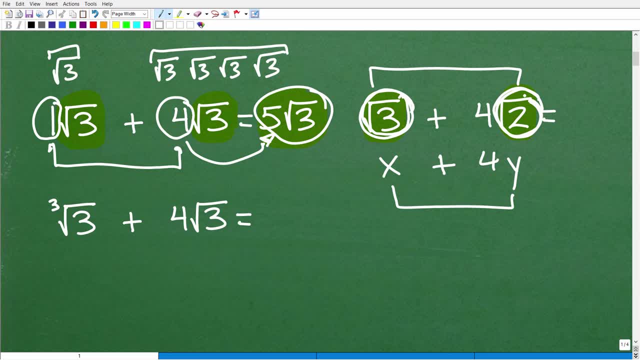 square roots. the square roots have to be exactly the same, exactly exactly the same. so let me erase this here, so we can see this crystal clear. okay, and i know this is a little bit confusing, but i'm trying to teach you this, uh, pretty quickly and uh, so let's go ahead and take a look again. 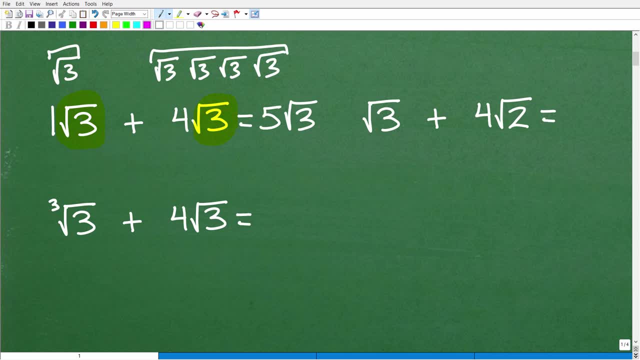 i can add these square roots or subtract them, because these this is a square root of three and this square root is exactly the same as this square. they're both square root to three. so i can do something with that and i just simply add or subtract these numbers outside of the square root. 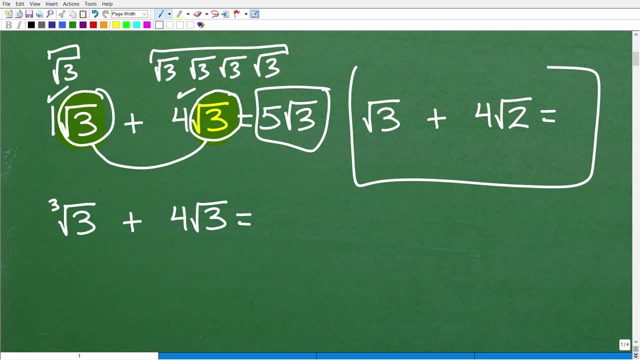 okay, again five square root of three. but in this example here, okay, i have a square root of three, so i can't do anything. i can't do anything, so i can't do anything. you know, matter of fact, all i can do is just leave it as it is, okay. so this right here isn't uh, is basically one kind of. 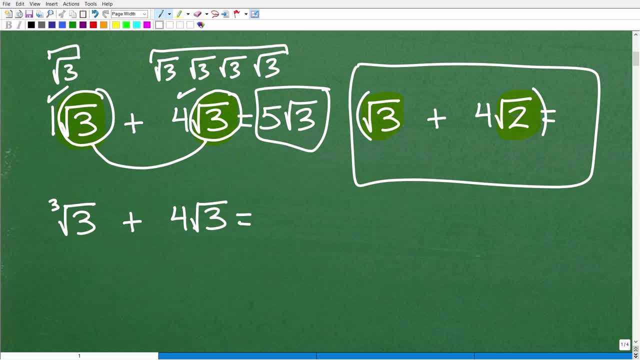 value. okay, one expression just like that, okay. so let's go ahead and take a look at this uh problem. so we have the cube root of three and the square root of three, right here, four, square root of three. so can i do anything with this problem? no, you cannot, because this is the cube root of three. this. 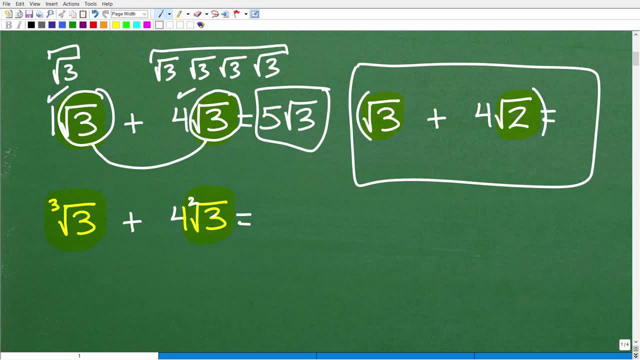 square root of three, and the square root is actually a little tiny, invisible, two up there. so, um, when you're adding and subtracting, okay, these have to be perfectly 100 percent the same. we can't have the cube root and the square root, but if we had the cube root of three, 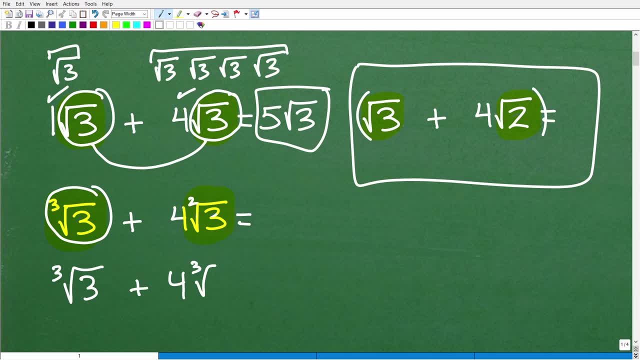 plus four times a cube root of three, or four cube root of three. we can do this because these are exactly the same. okay, so this would be again. there's a one outside here- this would be five cube root of three. okay, so we are talking about square roots, but i wanted to really, you know. 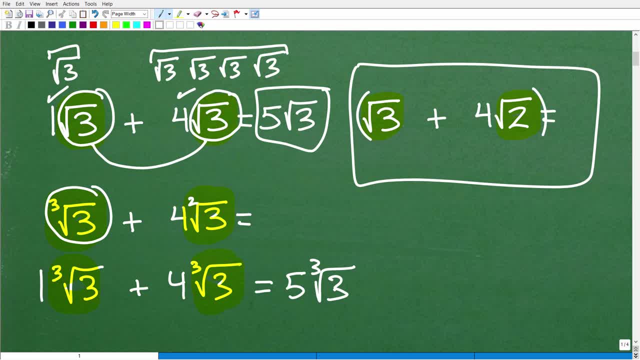 highlight, uh, two situations where you know, students can easily get a little confused about this. so, if you understand this, we can add or subtract square roots, but the square, the square root parts have to be 100 percent identical. okay, so let's go ahead and take a look at this next problem. here all 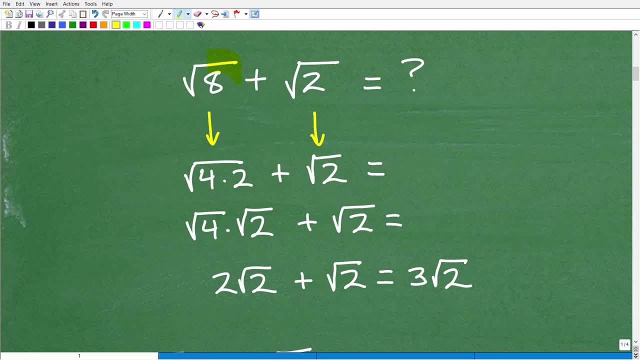 right. so here we have the square root of four plus the square root of two. so some of you out there might be like, okay, the square root, i'm sorry, the square root of eight, not the square four. here i have the square root of eight plus the square root of two. you're like, whoa, we can't do. 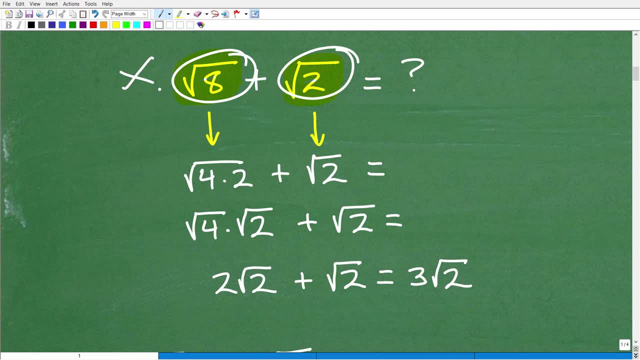 anything here, because these are not the same. so i'm going to skip this and turn in my quiz or test early and move on to i don't know, playing some nice video game on my cell phone. no, no, don't be in such a rush, because we can't really see the whole story here, the way this is written i have. 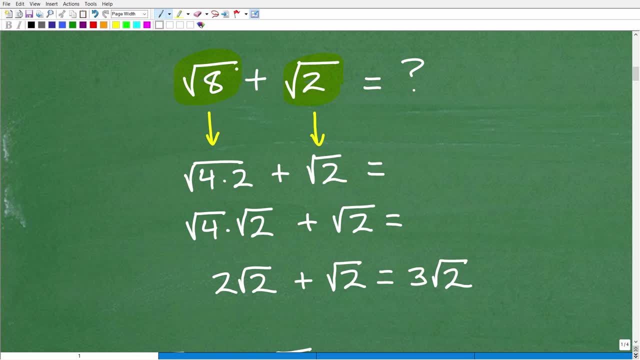 the square root 8 plus the square root of 2. what you need to do is you need to fully simplify all in order really to kind of see the reality of what's going on. okay, so i can't really uh assess whether i can add or subtract these two square roots here, because this is not fully simplified. 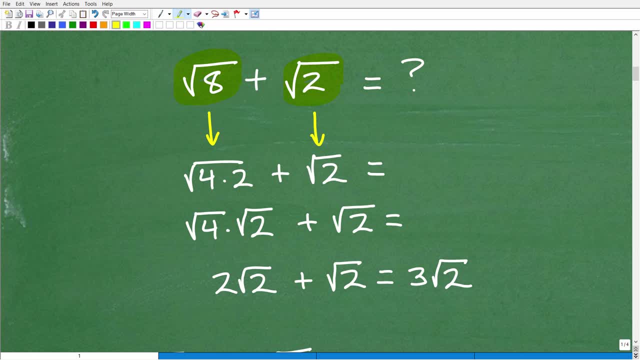 okay. so we're going to try to fully simplify it, and what i mean by this is we want to break this up in its factors. now, this is a separate video. i've been doing some other videos on square roots, so you need to know how to simplify square roots so we can write the square root of 8. 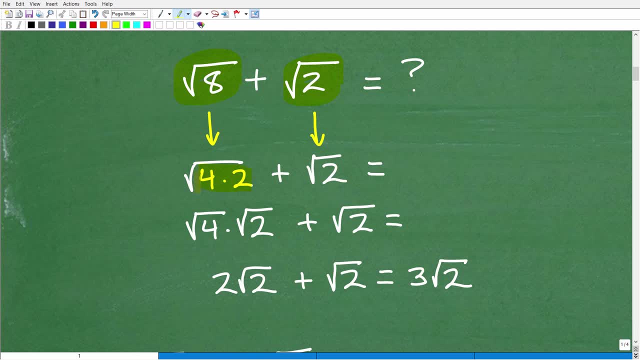 as the square root of 4 times 2. 4 times 2 is 8, and i could pull apart this one big square root into two separate square roots. so this is, uh, the same thing as the square root of 4 times the square root of 2, that is, the same thing as the square root of 8. okay, but the advantage of doing this? 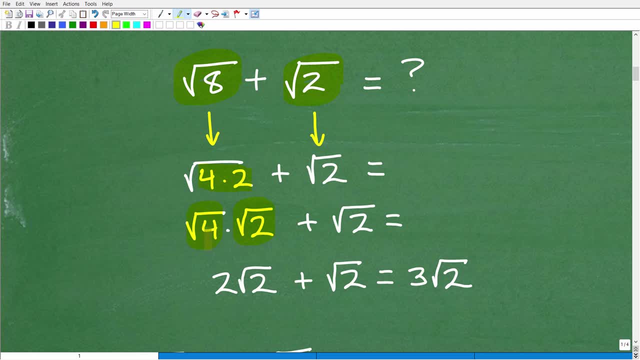 is the square root of 4. the principal square root, which is just the positive version of it, is 2.. so now the square root 8- really in a more simplified manner, can be written as 2 times the square root of 2. now i can look at this problem okay. instead of looking at this way, i can. 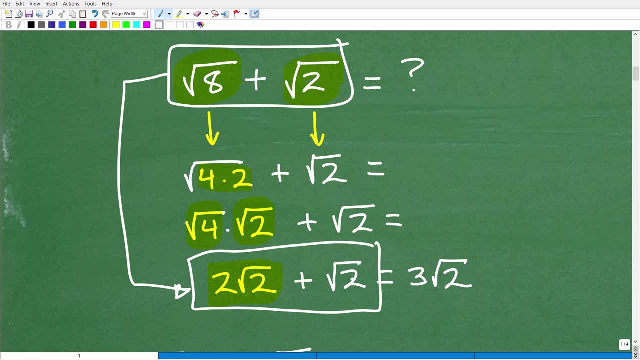 look at this way. okay, so this is 2 square root of 2 plus the square root of 2, and i can do this problem now because i have the exact same square root. okay, so this is 2 square root of 2 and there's. 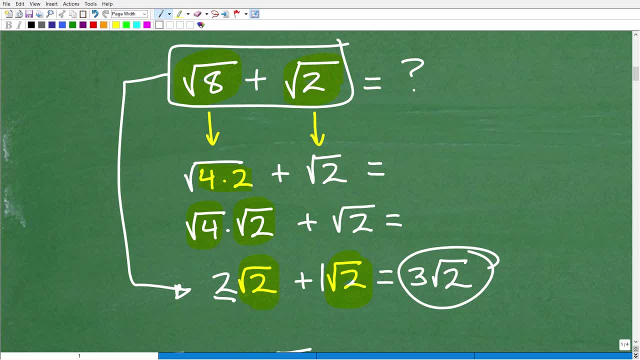 a 1 right here, 1 square root of 2. so how many square roots of 2 do we have? well, that would be 2 plus 1 or 3 square roots of 2.. all right, so hopefully you're getting a feel for this again. 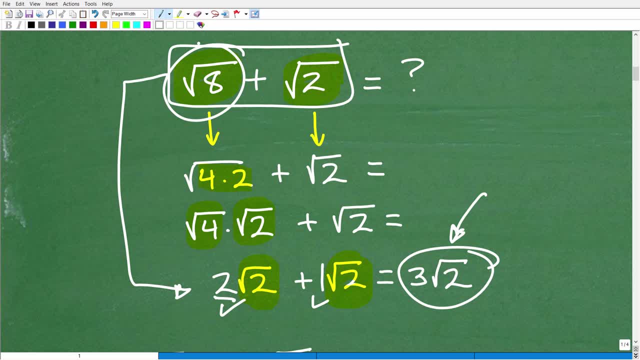 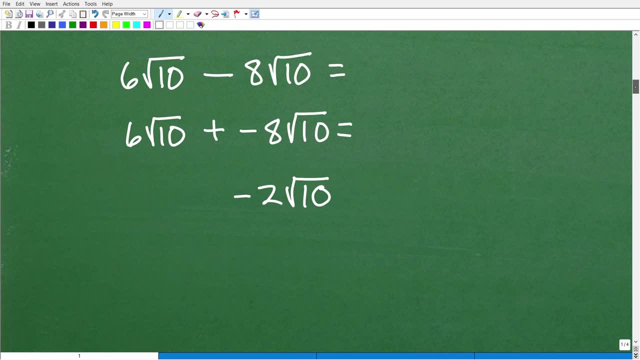 you're going to need to know how to simplify square roots, to add and subtract square root expressions. but let's take a look at a subtraction problem here real quick, because this is adding and subtracting square roots. so let's take a look at 6 square root. 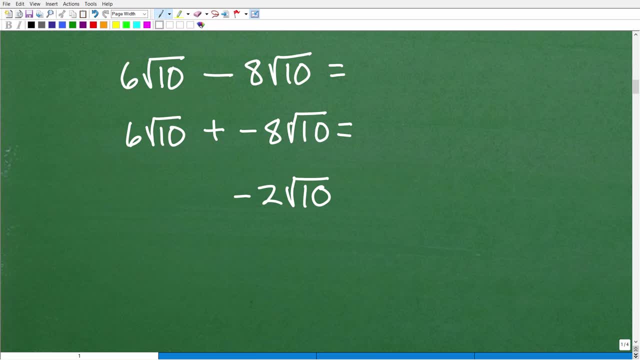 of 10 minus 8: square root of 10.. so how can we deal with this? well, first thing um first things first. we're looking at the square root of 10 and i'm saying, okay, are these the exact same square roots? they are square root of 10 and square root of 10.. so now you can just think of this. 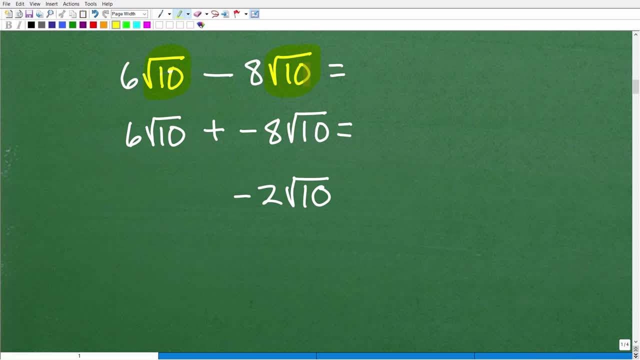 problem. as 6 square root of 10, minus 8 square root of 10, i could just write this as plus negative 8. this is a negative 8 there, okay, so i'm going to add these numbers- 6 and negative 8, okay, and i'm going to put that result in front of the square root of. 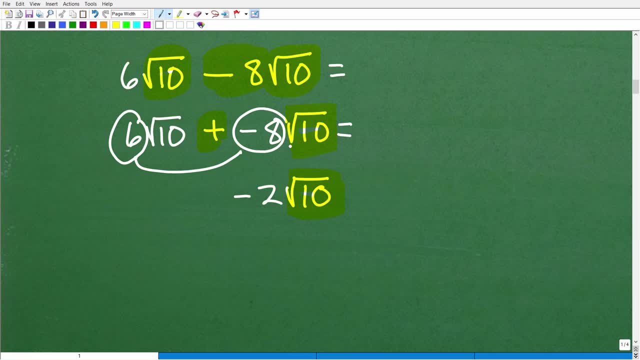 10. so 6 plus negative 8- hopefully you're up to speed on your positive negative numbers- is negative 2.. so the answer is negative 2 square root of 10.. now there's a lot of different uh problems here and additional practice and we can make this much more complicated. but if you 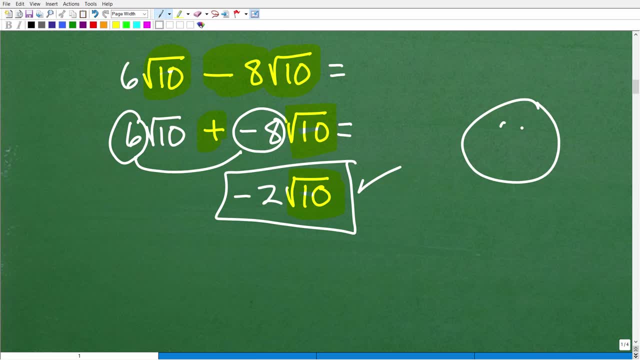 don't know the basics here and you got all this right. well then, let me go ahead and go ahead and give you a nice smiley face for, uh, just being a superstar in mathematics. let's get you an, a plus and 100. nice job now. generally i kind of put in some nice hairstyles, but we'll kind of skip that.